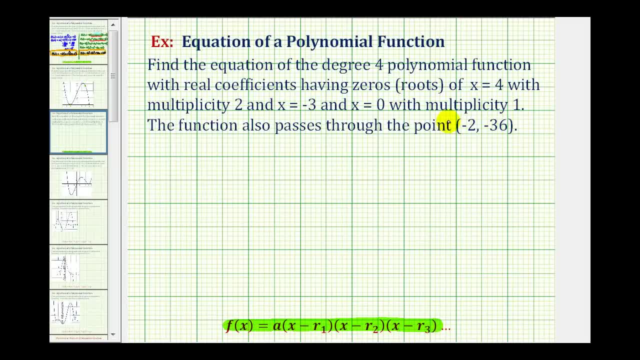 of our polynomial function, and then we'll find the value of a using the given point. So we'll start with f of x equals a times a factor of. well, the first zero is positive four, so our factor would have to be x minus four. 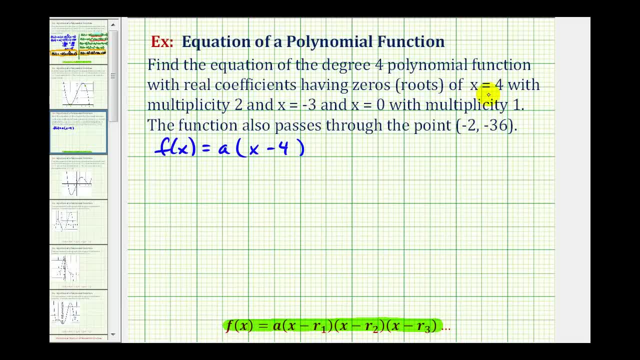 Notice: this zero has multiplicity two, which means x equals four, is a double zero. so we'll have two factors of x minus four, or we can just say the quantity x minus four squared. Notice: if we substitute four for x, this factor would be zero, making the function. 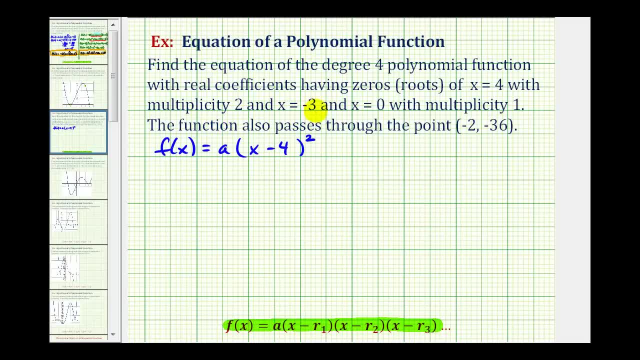 value equal to zero. The next zero is x equals negative three. so we'd have to have a factor of x minus negative three, which is x plus three. This has multiplicity one. so we have one factor. Notice if we substitute negative three for x. 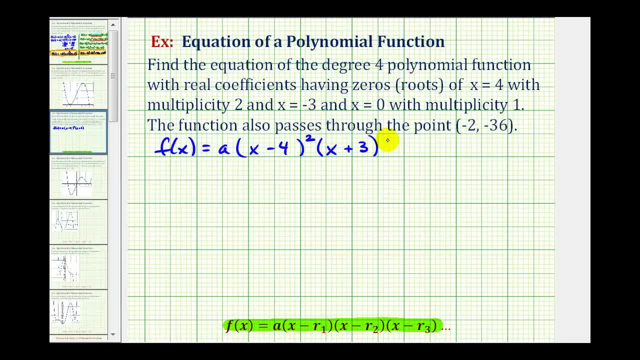 this factor would be zero, and our last zero is x equals zero, so we'd have a factor of x minus zero. Now let's go ahead and clean this up: X minus zero is just x, so we can write this as ax. 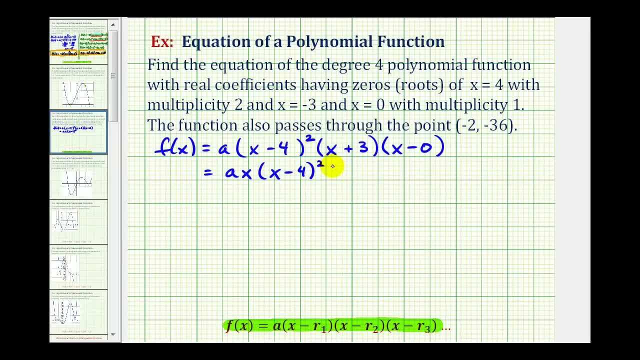 times the quantity x minus four, squared times the quantity x plus three. Now let's find the value of a, and we can do this using the given point here. If the function contains the point negative two, negative 36, that means f of negative two. 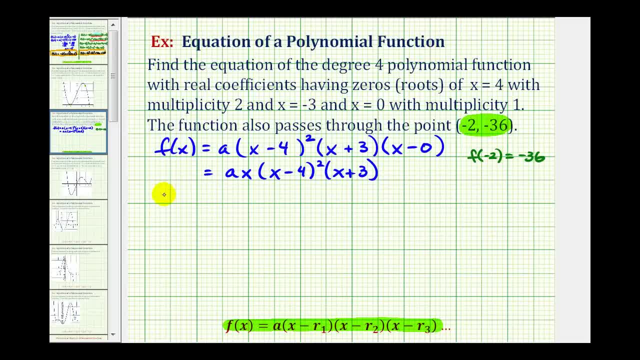 must equal negative 36.. So let's find f of negative two by substituting negative two for x, and then we'll set this equal to negative 36 to find the value of a. So we would have a times negative two or negative two. a times this would be negative two. 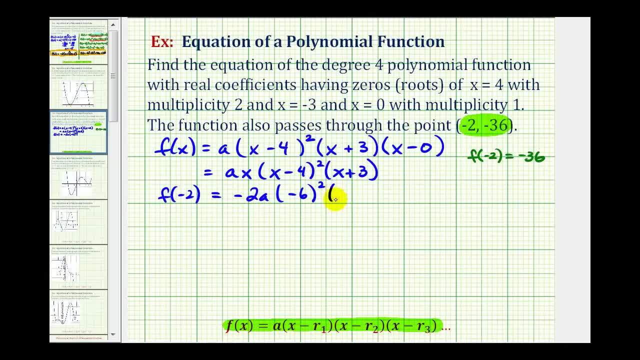 minus four, that's negative six squared, and here we'd have negative two plus three, that's positive one, and this must equal negative 36.. So we have negative two times a times positive, 36 times one, that's going to be negative. 72a equals negative 36,. 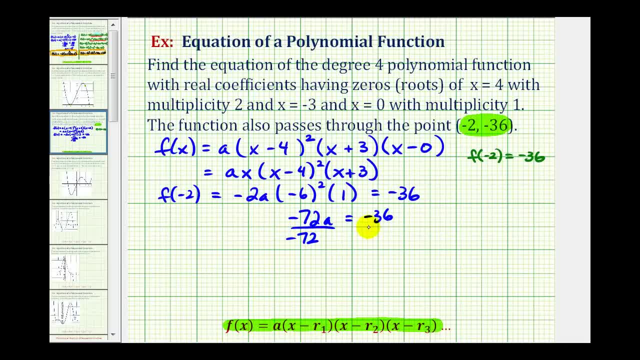 divide both sides by negative 72, and we have a equals positive 1 1⁄2.. So now that we have everything in factored form, our polynomial function will be f of x equals. let's go ahead and use this form here. 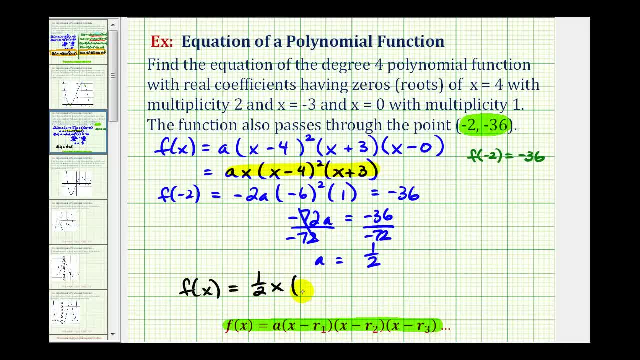 so we'll have 1 1⁄2 x times the quantity x minus four, squared times the factor of x plus three. This would be our degree four polynomial function that has the given characteristics. Let's go ahead and verify this graphically. 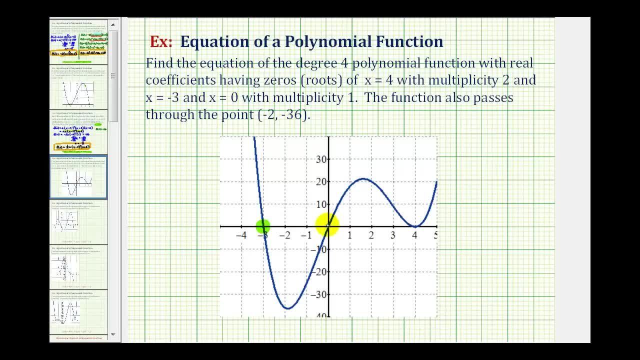 Here's our zero, or root of negative three and zero. Notice how the multiplicity is odd or equal to one, so the function crosses the x-axis. and then over here at positive four. notice how the function only touches the x-axis. 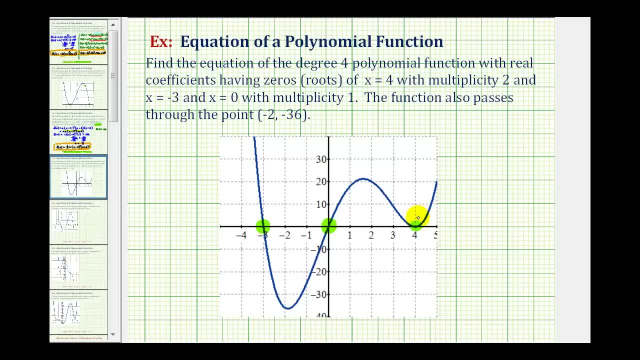 it doesn't intersect the x-axis. This is how a function behaves when the multiplicity is even. So the zeros, or roots, of this function look good. and if the last verification, let's make sure this function contains the point negative two, negative 36.. 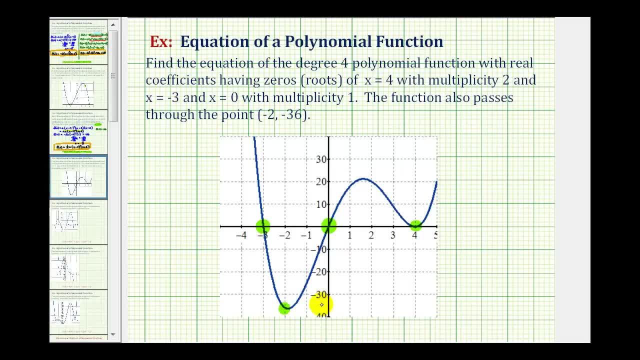 So here's our point: when x equals negative two and the y coordinate or function value does look like, it's equal to negative 36, so this graph verifies that our work is correct. I hope you found this helpful. Thank you. 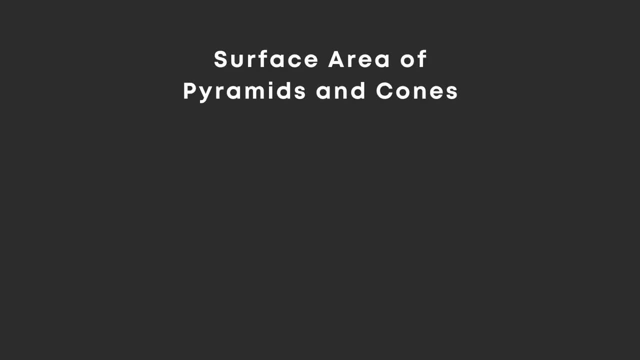 Hey everyone. Today we're going over how to find the surface area of pyramids and cones like these. If you also need help with finding the surface area of prisms and cylinders, be sure to check out my other video here. Let's go. 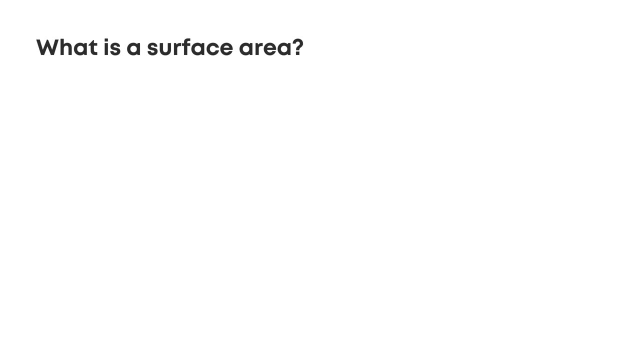 Before we jump into the problems, let's first review what the term surface area even means For a 2D shape like a triangle. all of the space on the inside of the shape is called the area. right, You can physically take a pencil and color in the area of this triangle.